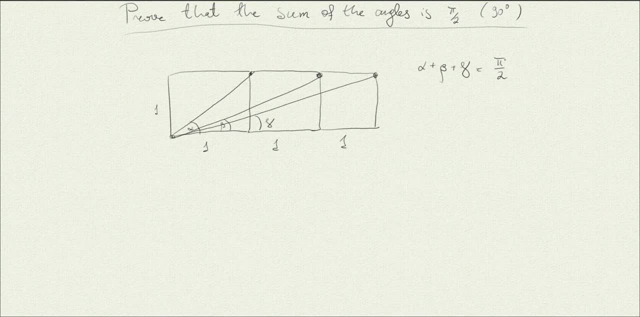 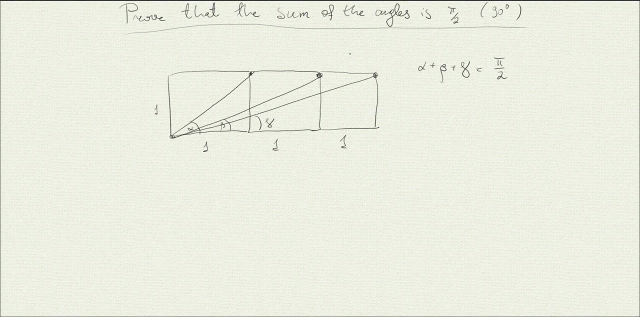 equal to pi half radians or 90 degrees, And if you try to prove it with Euclidean geometry it is possible. You need to do some clever constructions here, but you know it requires some work and it's not that trivial. I mean you can try, but it's not that simple And I would 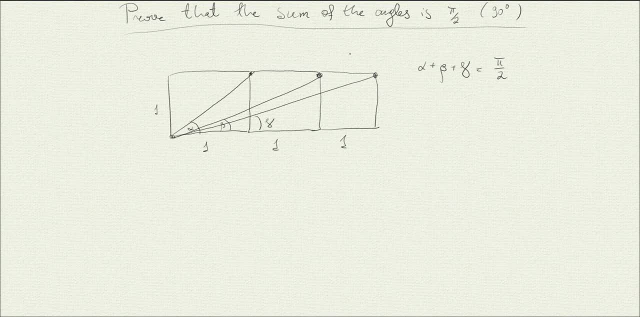 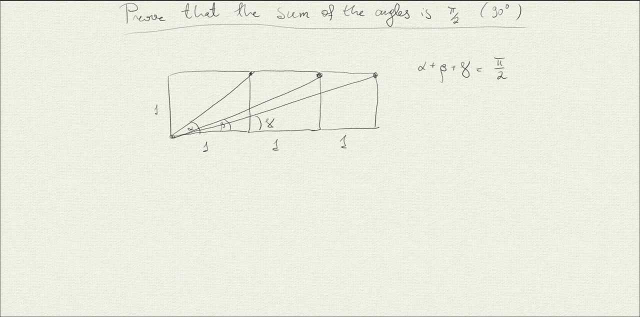 like to present here another way to look at the problem that will make this proof quite easy. So we can see right away that alpha is 45 degrees or a quarter of pi radians. but then it's equivalent to proving that beta plus gamma is pi quarter, which is not that simple, But there is a reason. 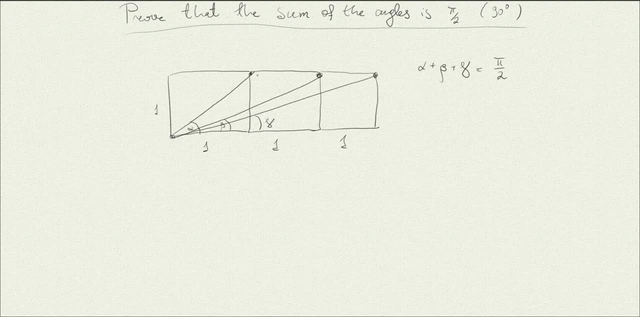 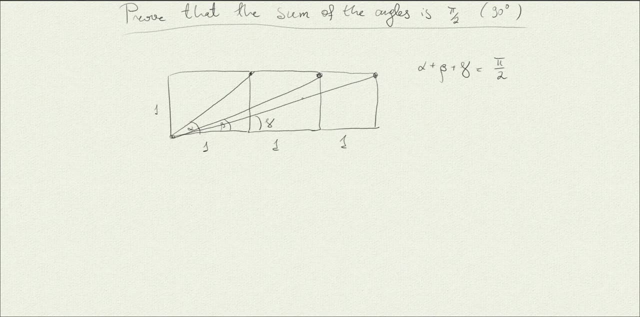 for this alpha here, But because the way I'm going to prove this problem is going to show that it's actually more convenient to think about it this way, And trying to compute it with trigonometry, like if we think of this as being 1, and this is 2, right, So it's like proving that arctangents of half plus arctangents. 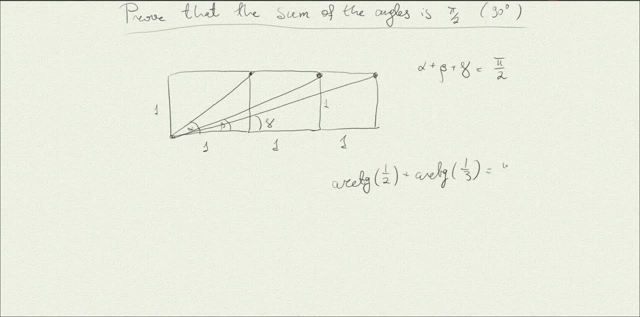 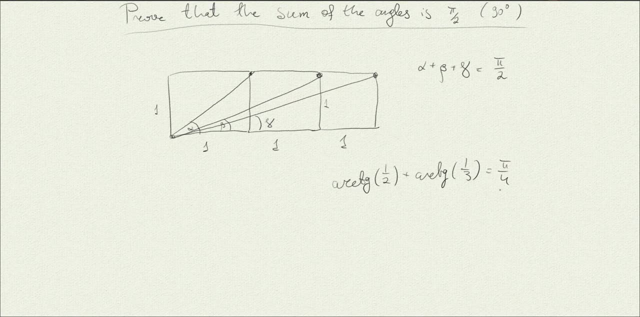 of one third is pi quarter. So this will be. this is not considered the proof, because you cannot verify it to infinite accuracy, But this will be a corollary from our proof. So let's see how can we think about this problem. So, if we'll think of this as being embedded in the plane, right And 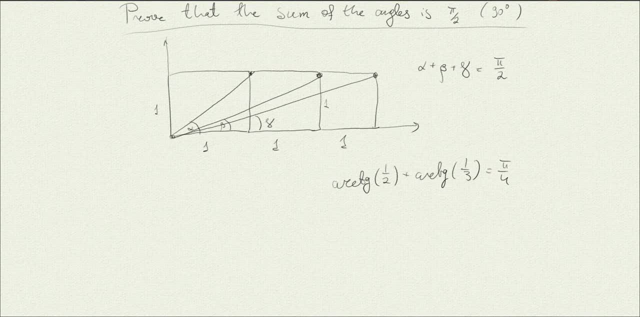 let's think of this plane as the complex plane, And the reason for the complex numbers will become apparent shortly. Then the coordinate of this point: this point is actually 1 plus i, and this point is actually 2 plus i and this point is 3 plus i. 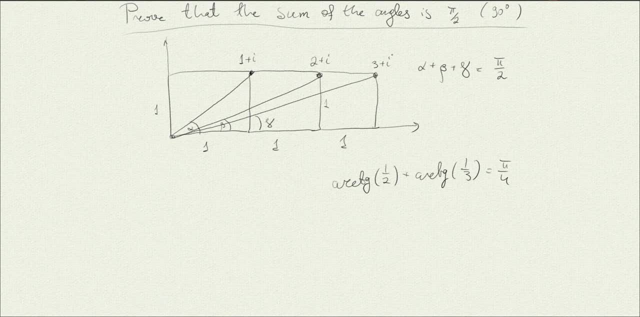 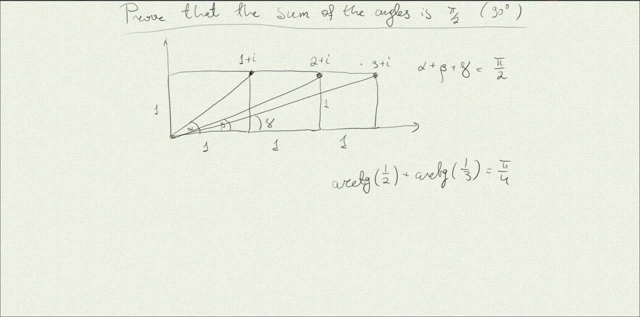 And we know that when we multiply complex numbers, magic happens. So when we multiply two complex numbers, their arguments are being added and their magnitudes are being multiplied. But if we think about it this way, then what we need to prove is that once we multiply all those, 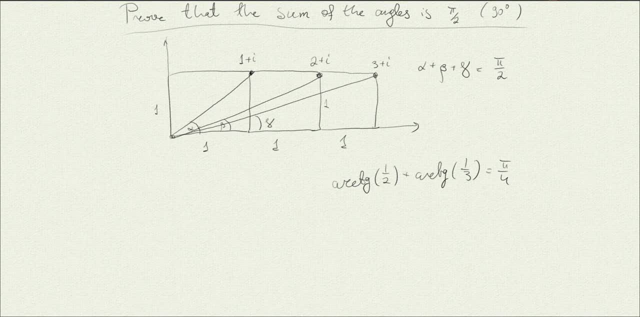 three numbers, we're going to be able to solve this problem. So if we think about it this way, then what we need to prove that once we multiply all those three numbers, then the argument of the result will be the sum of the angles alpha plus beta plus gamma. 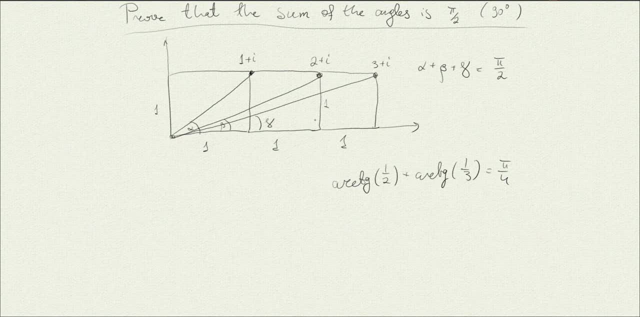 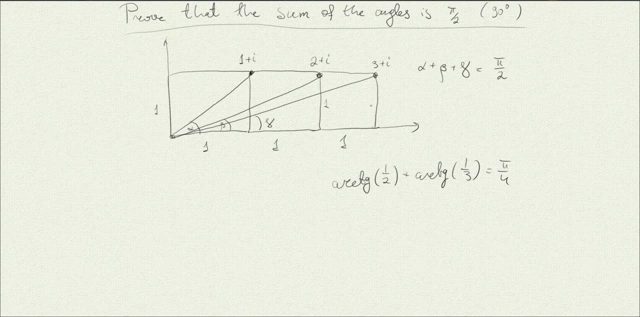 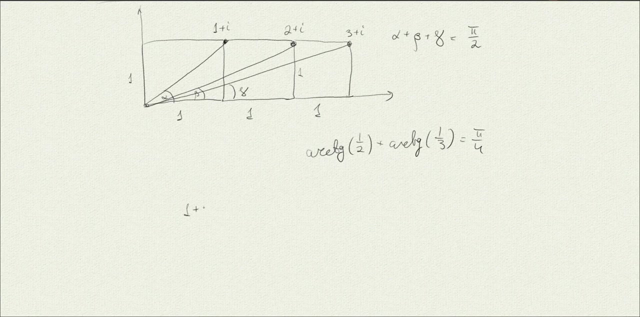 on the one hand, And so it's clear from here that it would be enough to show that the product of all those three numbers is a purely imaginary number, right with a positive imaginary component. So let us try and compute this. So, when we take 1 plus i, times 2 plus i, times 3 plus i, 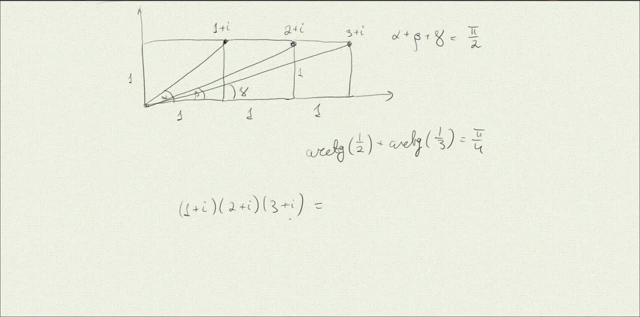 let's see what we get. So the argument of this number is alpha plus beta plus gamma, as I said, and let's multiply it. So what we get here is 1 times 2, and then minus i squared, which is 1,. 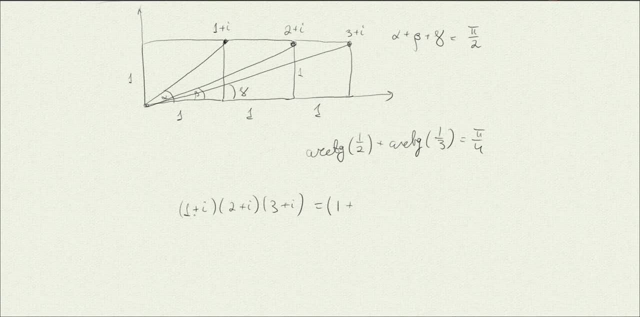 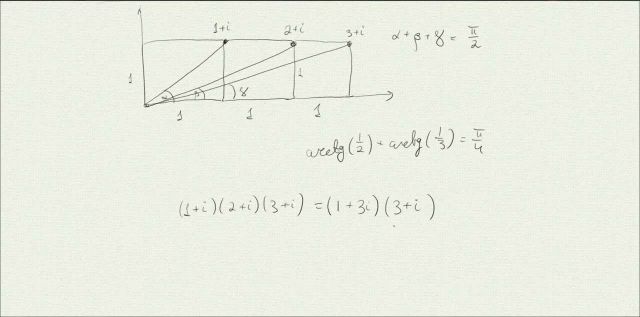 so it's going to be 1 plus. and then how many? i's 3i and times 3 plus i. Now, actually, we can see right from here- I'll prove it- that this number is going to be purely imaginary. but let's. 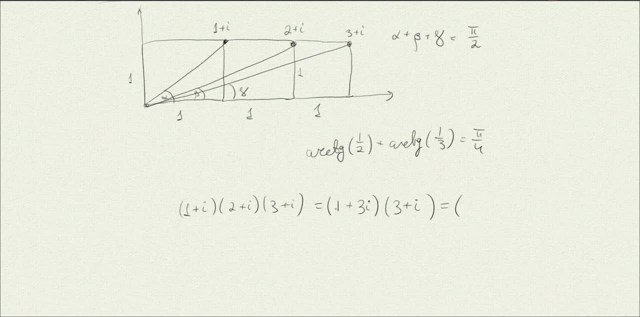 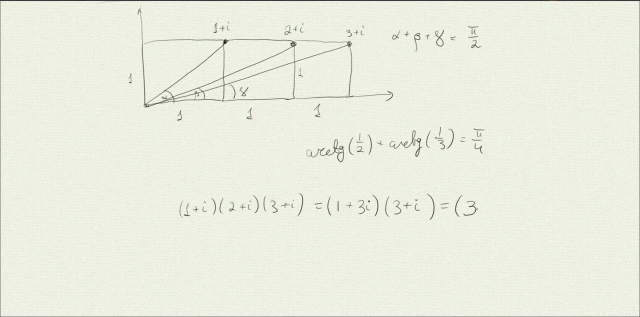 go on with the computation. So it's 3 times 1 times 3 is 3, and minus 3i squared is actually minus 3, that's the real part. and the real part as we can see here is 0, and the imaginary part. 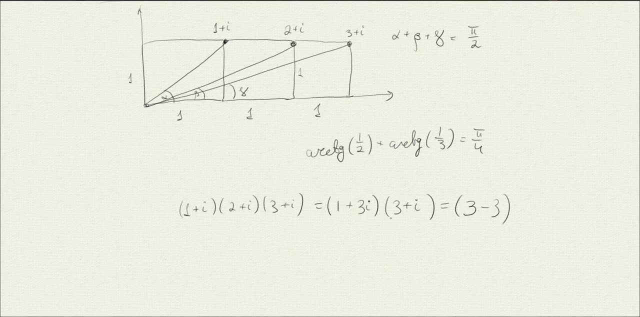 is going to be. then we're going to have 10i plus 10i. So, as a result, we get 10i and 10i on the imaginary axis is here, and then we're going to have 10i plus 10i. So, as a result, we get 10i and 10i on the imaginary axis is here. 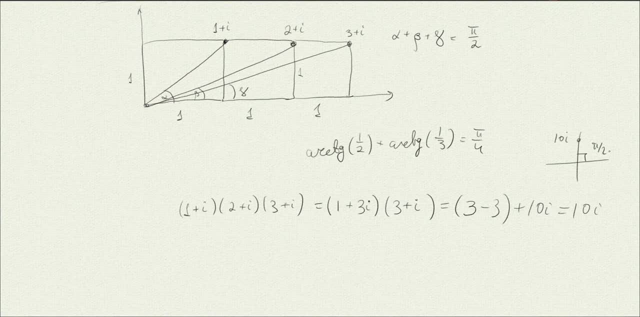 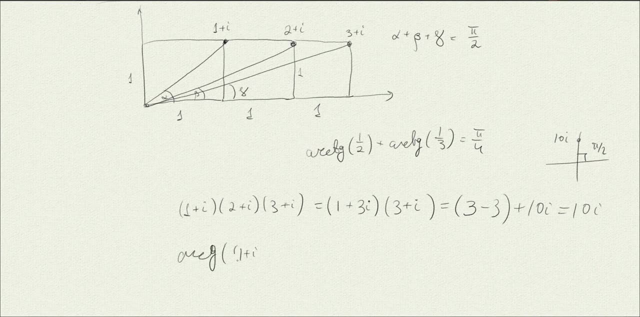 and its argument is pi half. indeed, Therefore, the argument of 1 plus i times 2 plus i times 3 plus i, it equals to alpha plus beta plus gamma. but it's also equal to the argument of 10i, which is pi half, and therefore, 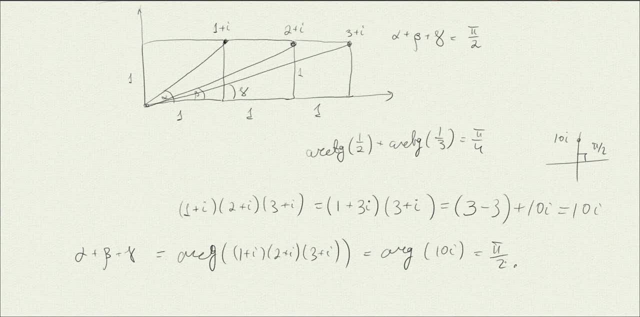 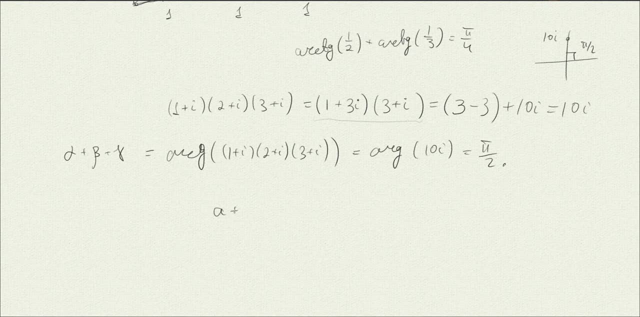 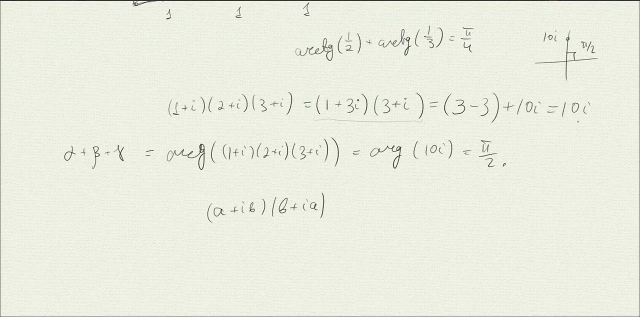 this problem is solved and this is proved. And one nice observation here, just a geometrical one. then: whenever we multiply a number- a plus ib, times b plus ia- we are always going to get a purely imaginary number because, as we have seen, it's going to have zero real part.